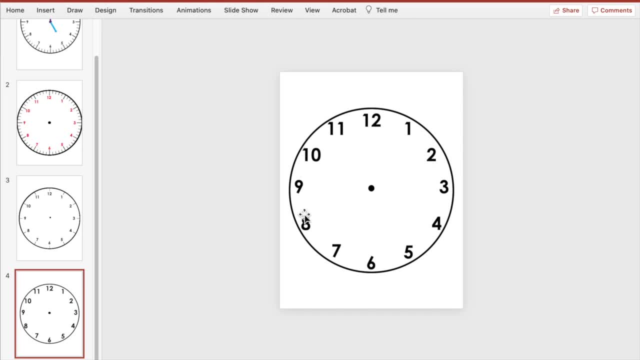 I'm going to show you how to create a basic analog clock just showing the hours. The second part: we will be adding in tick marks for our hours. The third part: we're going to add in tick marks to represent each of the 60 minutes. And in that final part, 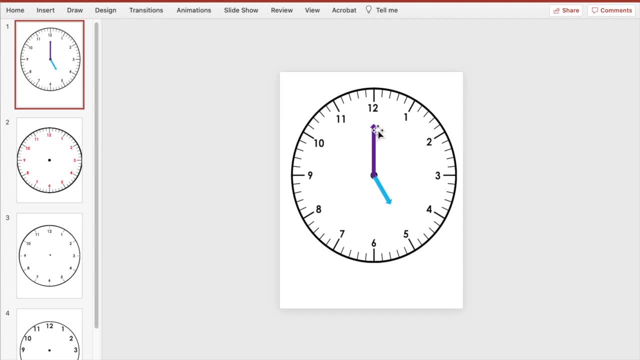 we're going to add in shapes to create an hour hand and a minute hand. If you want to skip ahead to any specific part, there will be timestamps for each part in the description box below. In this video I won't be showing you how to set up a page to be vertical. 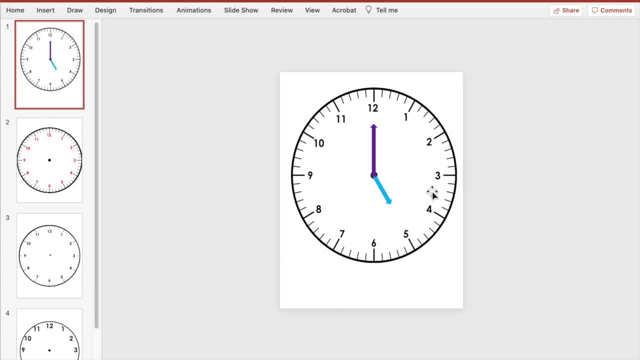 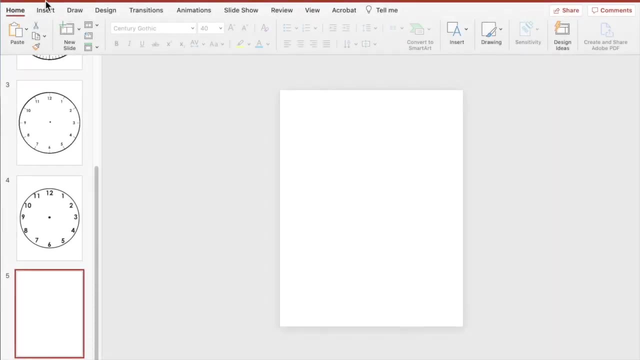 eight and a half by 11.. If you want to see that, check out any of my other how-to tutorials in the 30-day challenge. Any of the videos from 1 through 15 show you how to set up your page. For this first clock. we're going to start by. 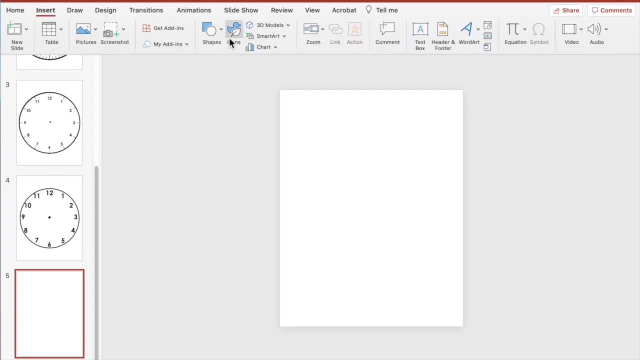 going up to insert and then clicking on shapes. We're going to choose this donut. You can find it under basic shapes. I'm going to click on my page and then hold the shift key down so that my donut stays proportional in its dimensions. I'm going to get it as large as I can And I'm 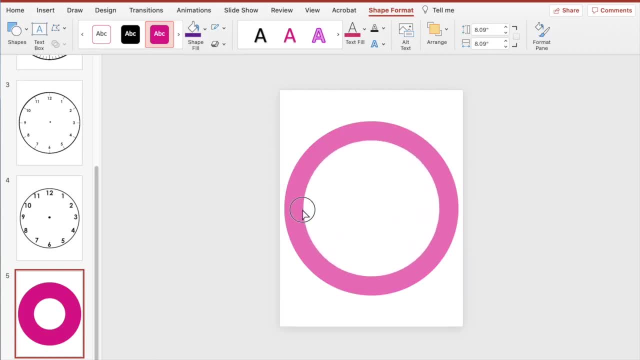 going to select the inside of the circle to thin out that border and then change it to black. So there's our outline. Now I want to add in our hours. I'm going to go to insert and go to text box. I'm going to create a text box. I'm going to type in that number 12 and go ahead. 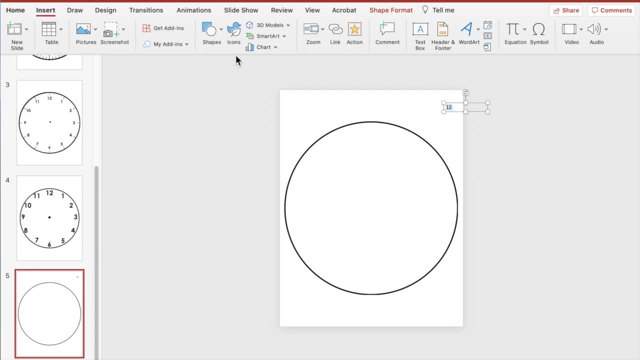 and change the font and size now. So let's go to home center it change that font and then make it a little larger. So I'm going to go to home center it change that font and then make it a little larger. 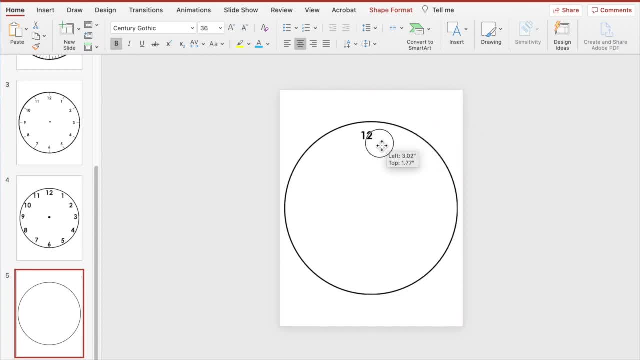 I'm going to go with 12 and then line it up with those grid lines and center it. I'm going to duplicate that to make my six. I'm going to duplicate that. I'm going to duplicate it twice so that we have the one nine and we can bring in that text box. Let's duplicate this one. 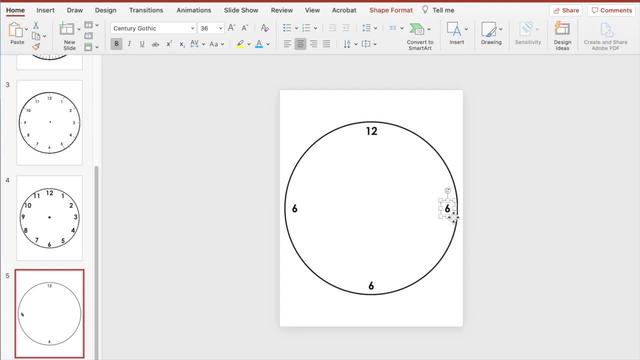 And we're going to change it to nine and we're going to change it to three, So then I'm going to duplicate the other numbers, All right. we're going to change our numbers out, All right, and then we're going to just make sure they're all in a good position. 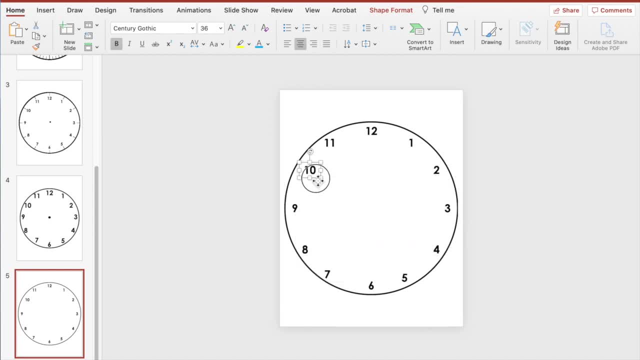 And then we're going to go ahead and create a text box. So let's go to home center it, change that font and then make it a little larger. And then the last thing we're going to do is add in a dot for that midpoint in the middle of our clock. 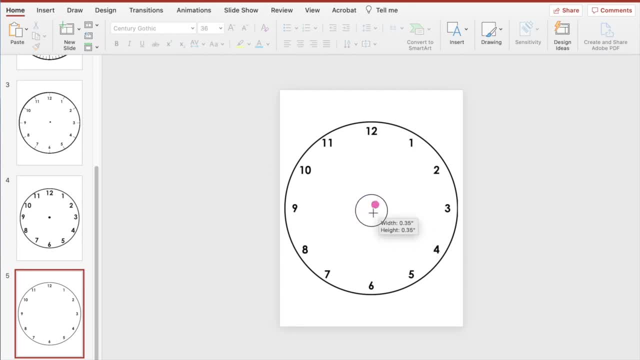 Again, I'm going to hold down the shift key so we don't change the shape of the circle, and then I'm going to center it And then change the fill color and make it have no outline. So there is our basic analog clock with just our hours. You can make the size of each number larger or smaller, based on however you prefer. 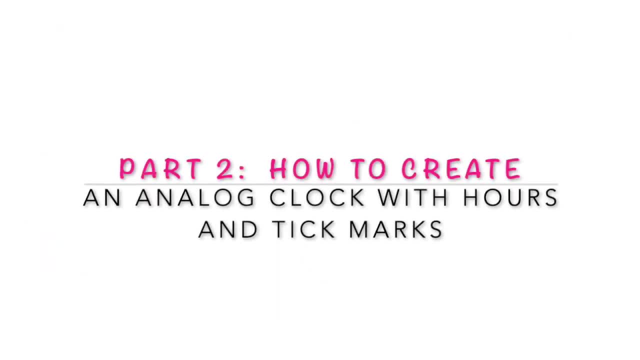 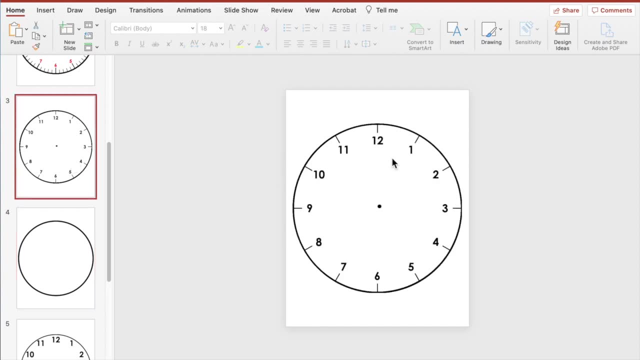